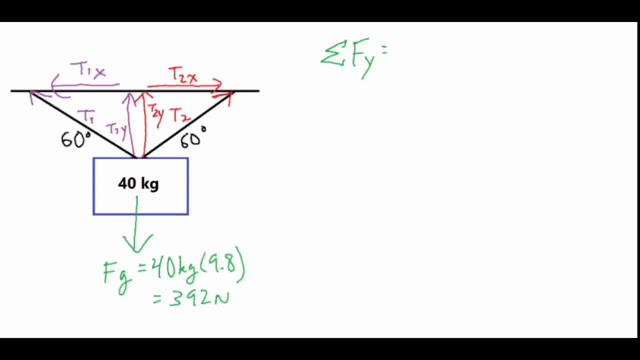 we'll call T1x. Now, if we're just analyzing the vertical components, we have two going upwards, so we'll call the T1y and then we'll call the T2y. So we'll call this one T2y and then we'll call this one T2x. 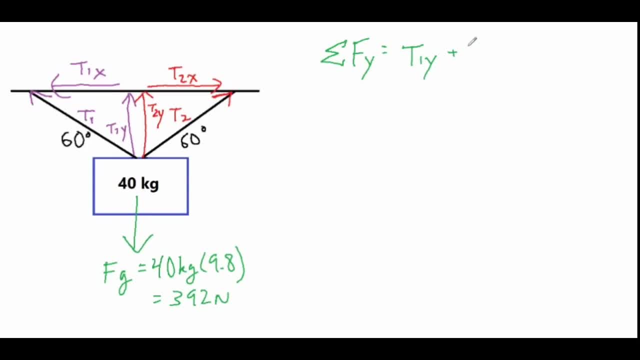 t1y positive and the t2y positive and then if you subtract the force of gravity that's going downwards, you will have no force because our object is at rest. so one thing we know is that we know that, because the angles are the same, that these two values are going to be the same. so we 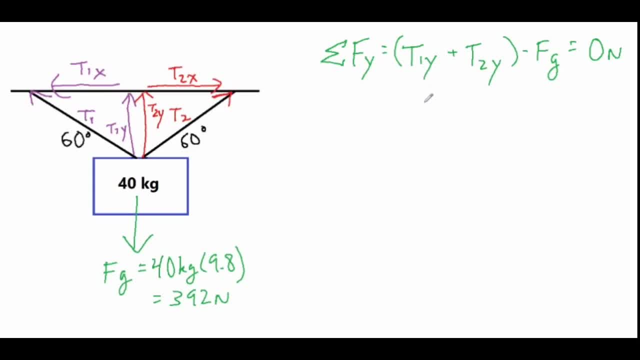 can go ahead and just kind of combine these two together and we'll call it 2 ty, and we won't distinguish if it's t1 or t2, because those are going to be the same anyways. okay, and then we're going to add fg to both sides, so that equals the force of gravity. 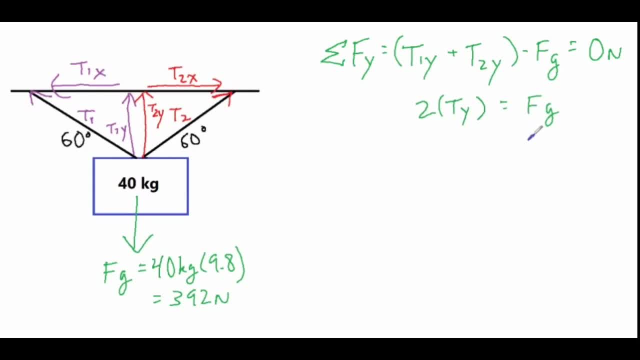 which we already know that value. anyways, that value is going to be 392 newtons. so basically we're going to split that force up and and divide both sides by two, and that our ty equals 196 newtons. now we could analyze these x components. it's actually not necessary in this problem. 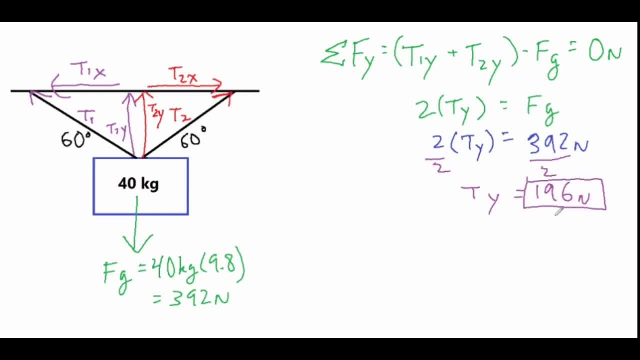 so as long as we have one side of our triangle, either our red triangle or our purple triangle, and we have an angle to work- with which we already do- we have a 60 degree angle- then we could just use some trig to find all the other components. now what we can do is we can use 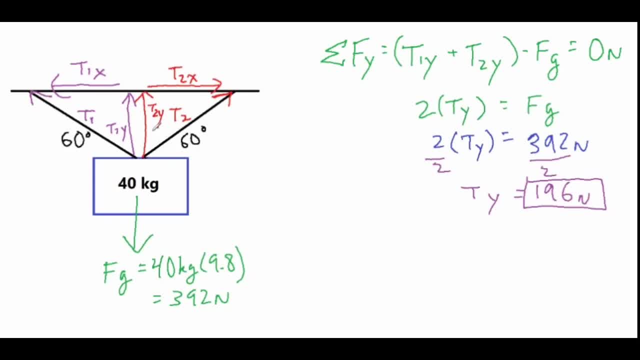 this triangle because there's a 90 degree angle here. if this is 60, then this must be the complement, which is 30 degrees. so i'm going to go ahead and use that 30 degree angle and i want the t2, which is the hypotenuse, and i have this component over here which is actually my adjacent angle, or. 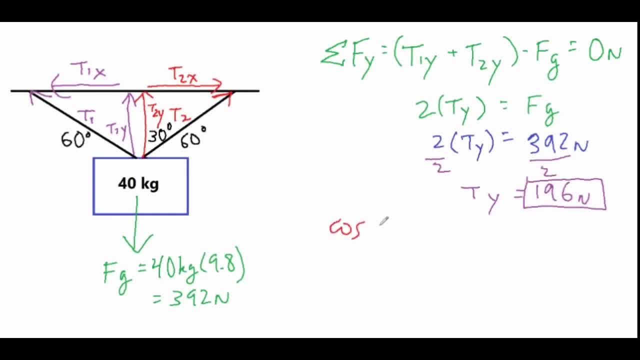 adjacent side, excuse me. so we have the cosine. cosine. cosine of 30 degrees equals the adjacent, which is the ty side, divided by the hypotenuse, which is the t2 side, and we already know this one is 196. so then what we can do is we can go ahead and cross.